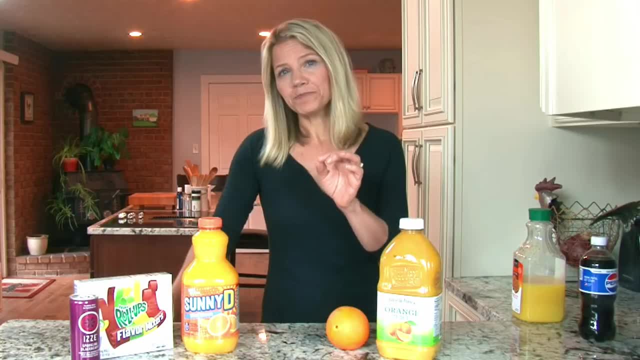 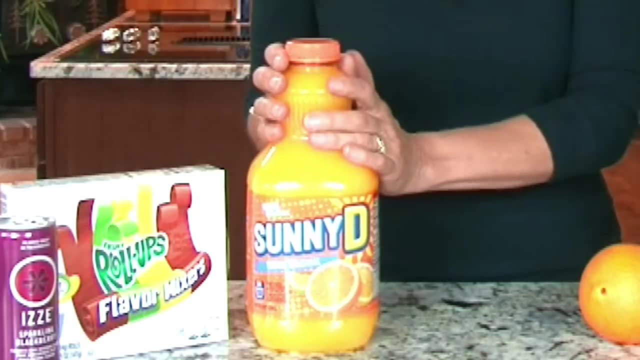 so I don't want to go too deeply into that here, But it did lead me to pick up a bottle of this Sunny D when I was at the grocery store, so I could point out the ingredients for you If we read the label. 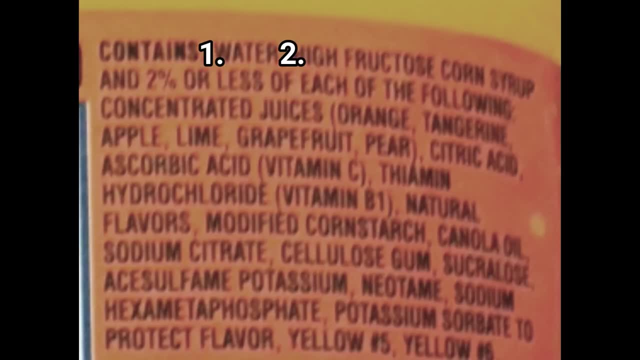 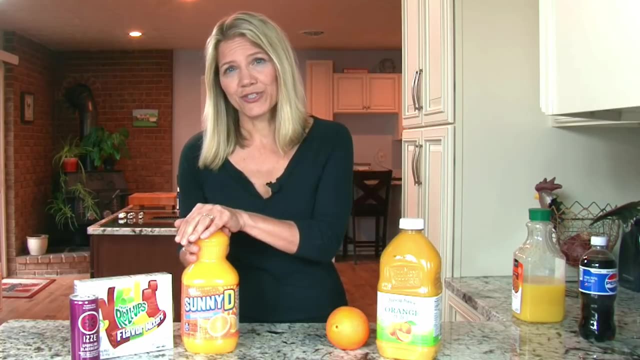 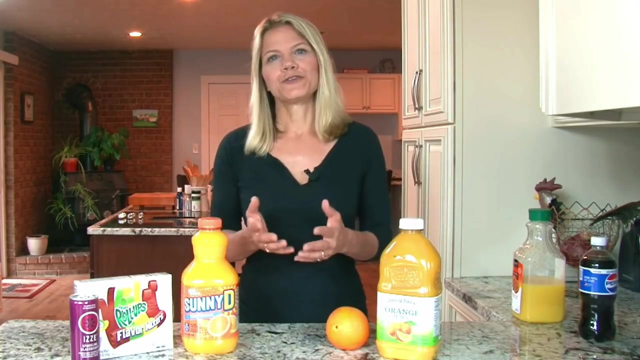 we see that the first ingredient is water, the second is high fructose corn syrup, followed by juice concentrates. There is nothing nutritious in here and it is simply sugar water. yet it is marketed as a sensible drink for kids, And it's worth noting that fruit juice concentrate is not only in fruit drinks. 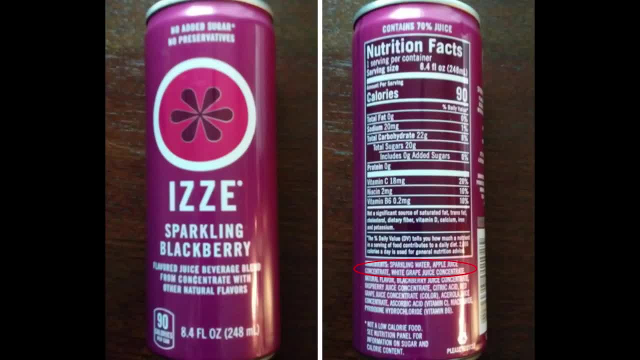 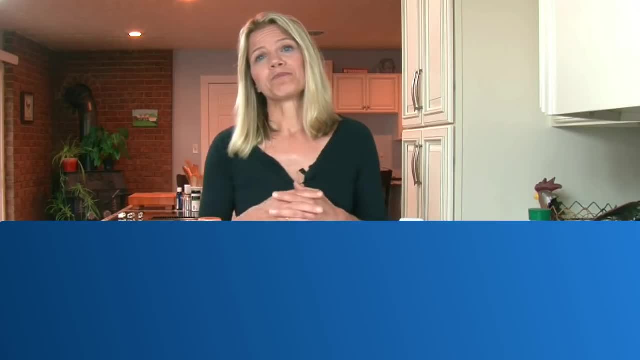 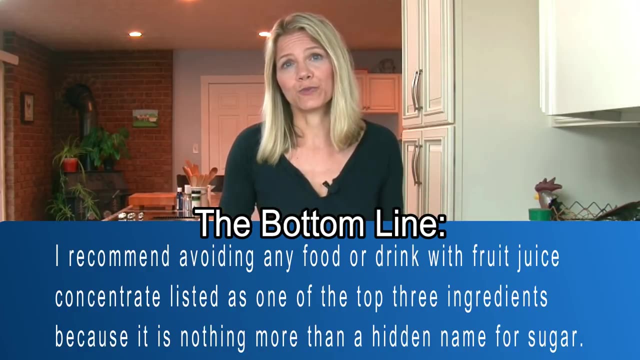 It is in many foods and energy drinks, So you need to read labels on snack foods and energy bars and energy drinks. So the bottom line is that I recommend avoiding any food or drink with fruit juice concentrate listed as one of the top three ingredients. 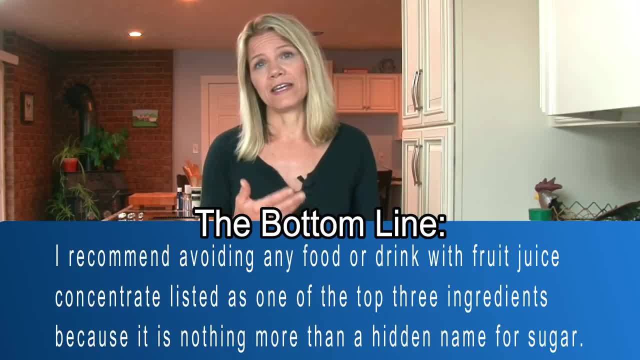 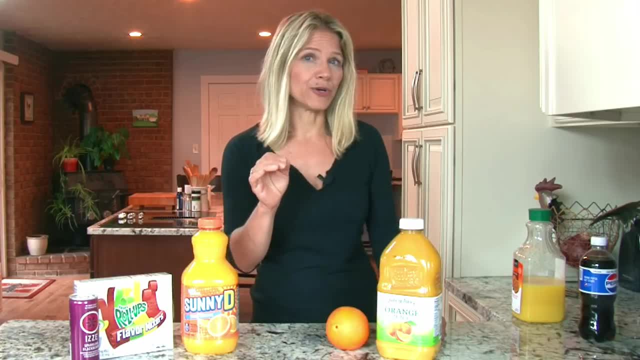 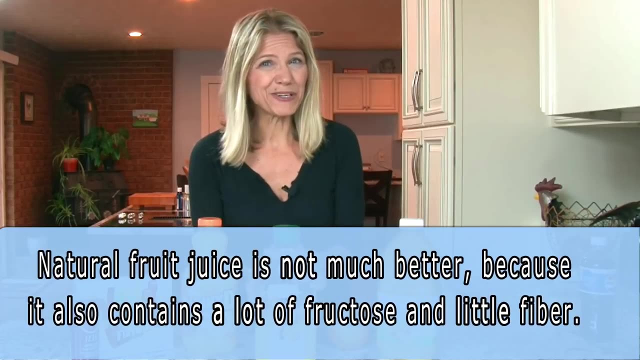 because, at the end of the day, it is nothing more than a hidden name for sugar. Now I do want to end with a brief discussion of natural or not from concentrate juice. I will say that drinking a glass of natural fruit juice is not much better. 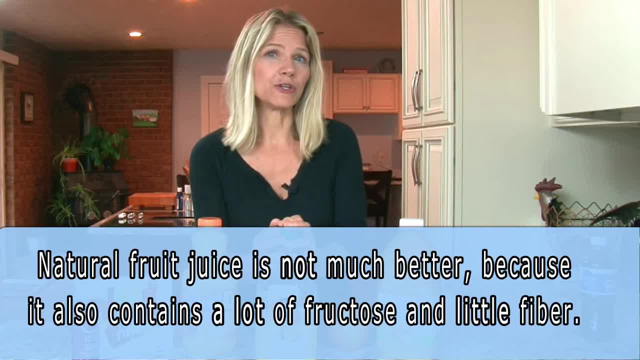 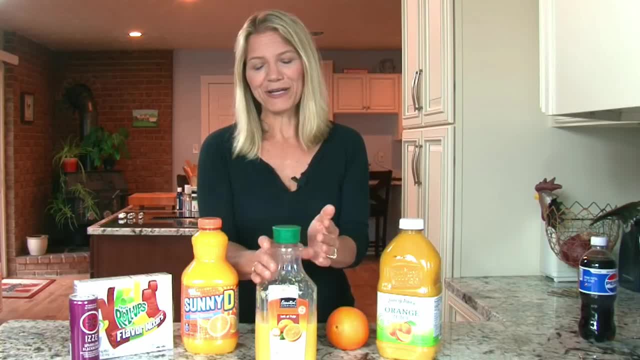 because that juice is going to put a lot of fructose into your body, much more so than you would have if you ate the whole piece of fibrous fruit. But I know somebody's going to comment and ask me why this fruit juice is half empty. 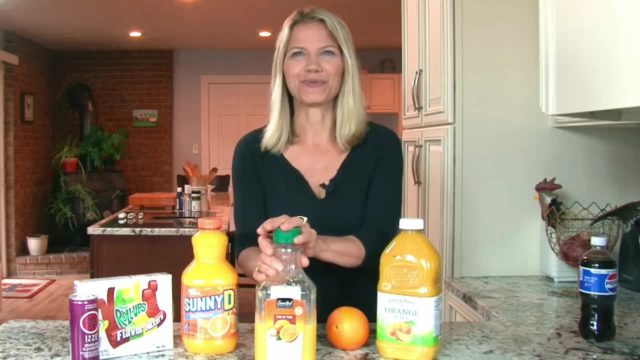 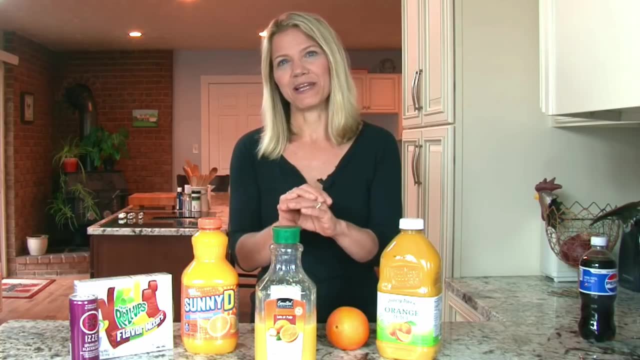 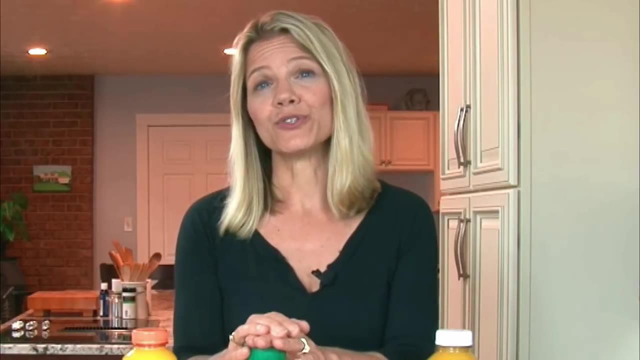 The reason is because I use about a third of a cup about three times a week in my smoothie as part of my enjoyable maintenance plan. So if you are not there at that point yet, you might want to leave the fruit juices go and go instead for the full fruit juice. 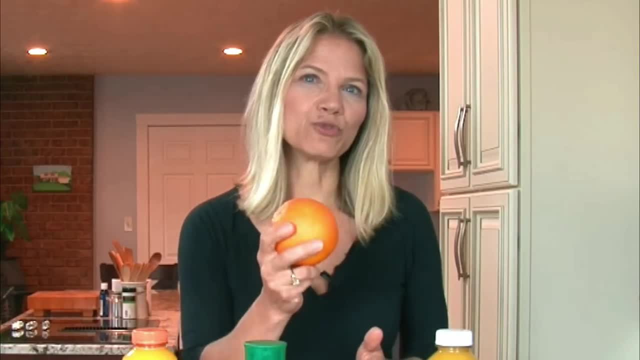 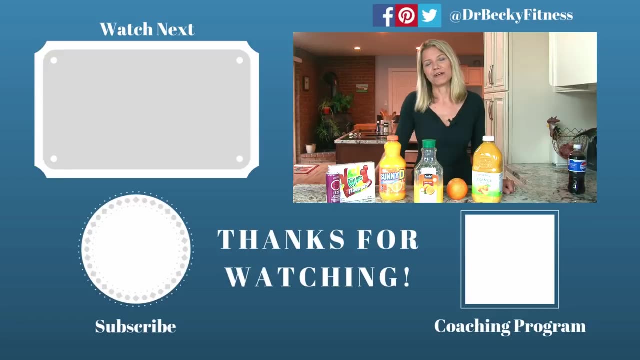 The fruit juice has a nice amount of fiber with it to control the absorption of that fructose. If you aren't at that point yet and you'd like some guidance on getting there, I invite you to check out my coaching program. But for now that is all I have to talk about. 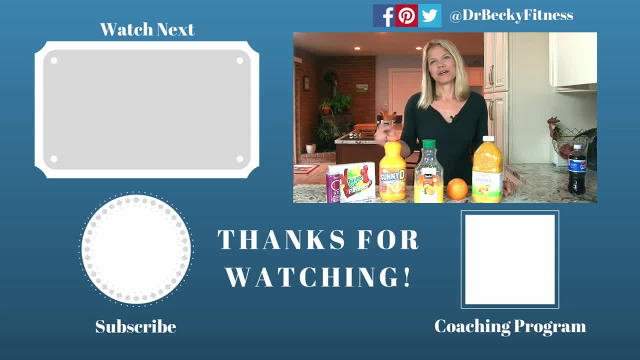 and I hope that you enjoyed it. If you did, please subscribe to my YouTube channel here, and I'll be back very soon with another video to help you reach your goal. Thanks,